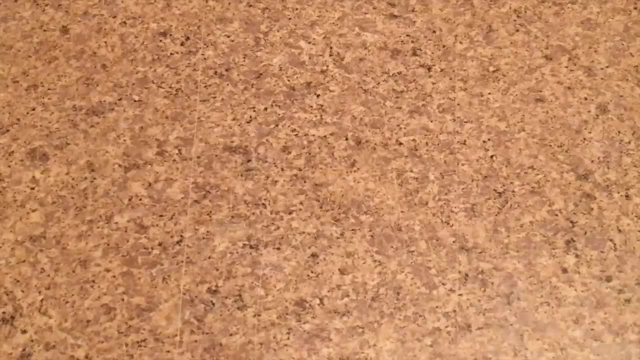 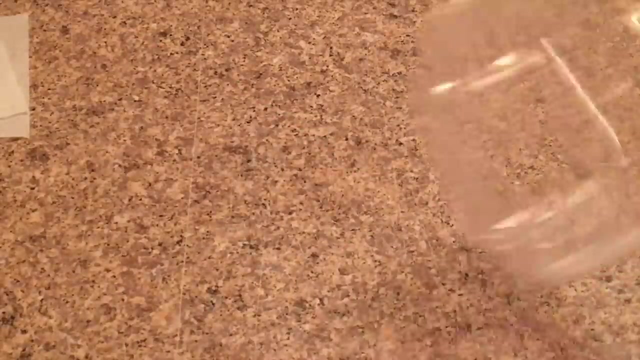 so the first no glue paper slime recipe I will be testing today is toilet paper slime. So the ingredients you guys will need to make this slime recipe today is dish soap. I'm using the Ajax dish soap. The next thing you guys will need is toilet paper and a bowl or plate to make your slime. 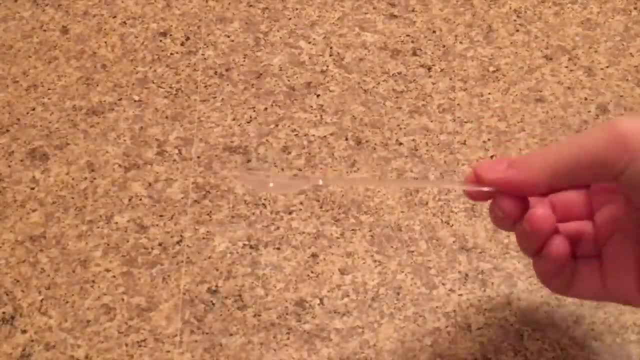 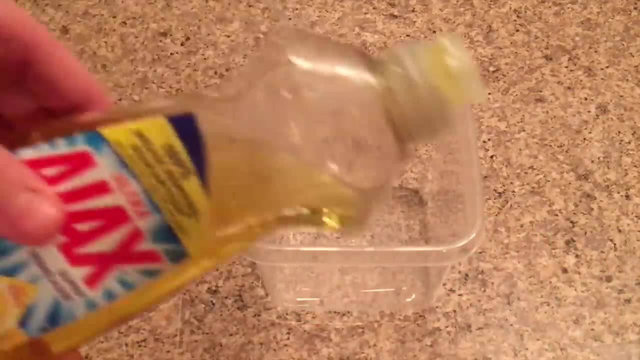 in And last but not least, you guys will need a mixing tool. So you first are going to have to take out your bowl or plate and add in your dish soap. And it's this kind I got like the lemon kind, because this one works really good for me. I tried it out before. 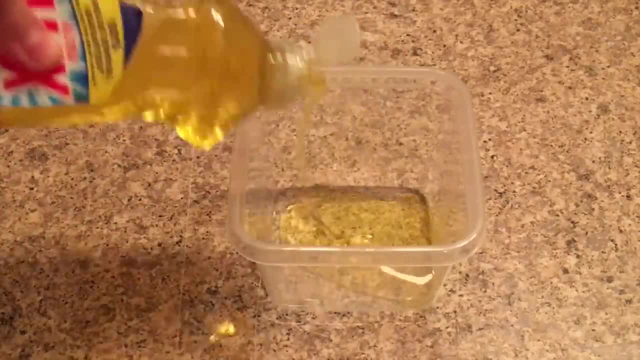 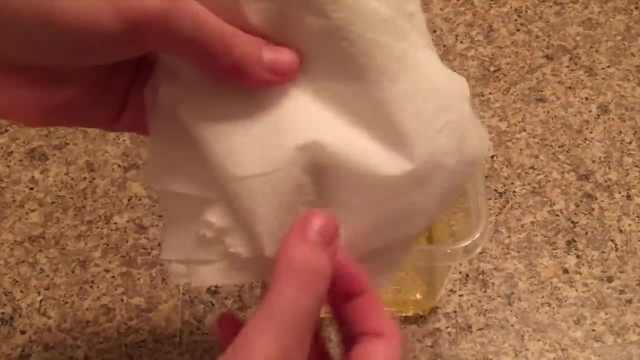 for like a no glue soap slime on my own and it worked really good. So I suggest using this type of dish soap if you want to, And add as much as you want into there. So I added that much And now you guys are going to have to add in your 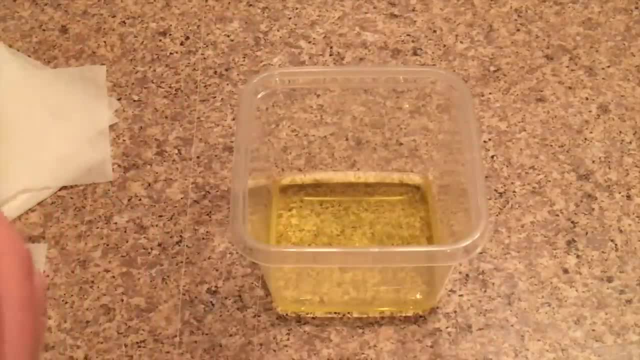 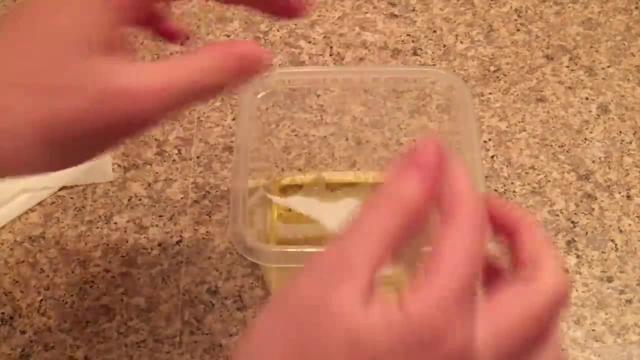 toilet paper And you guys want to rip it up because, like, if you keep it like I don't know, kind of like full, like it was before, it's going to get like all clumpy and it's not really going to turn into slime. So I suggest not doing that. So do what I'm doing. 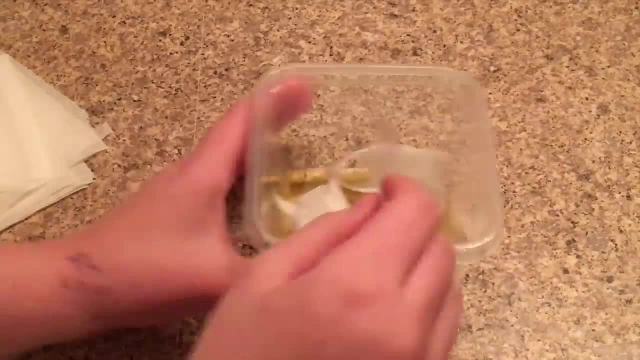 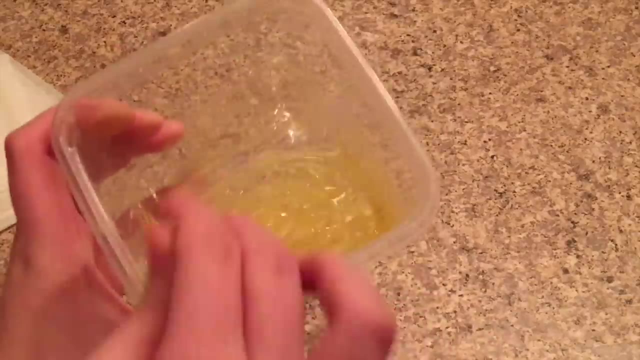 Just rip it up into little shreds And then after that you guys are going to mix it around and mix kind of like slowly But not too fast, because if you mix really fast it's just going to get all clumpy And 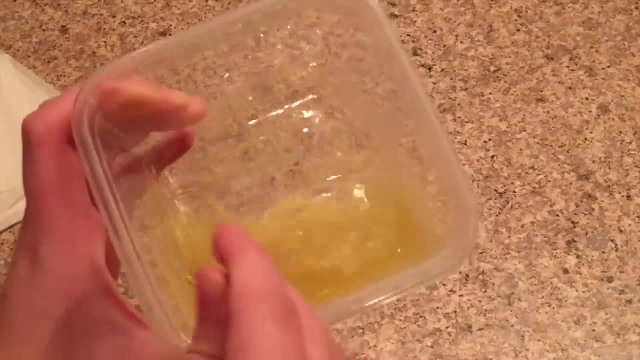 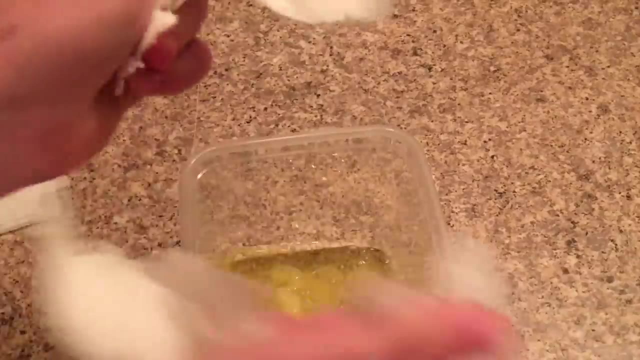 like you really don't want that. So just keep mixing it together. You can see there's like some little clumps, but that will probably dissolve. I'm going to add in a little bit more because I kind of want to give it a little thick, or. 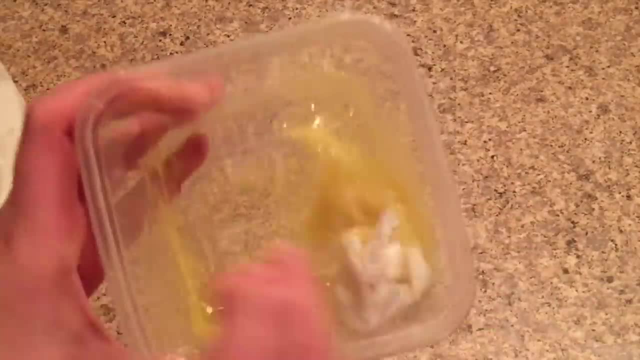 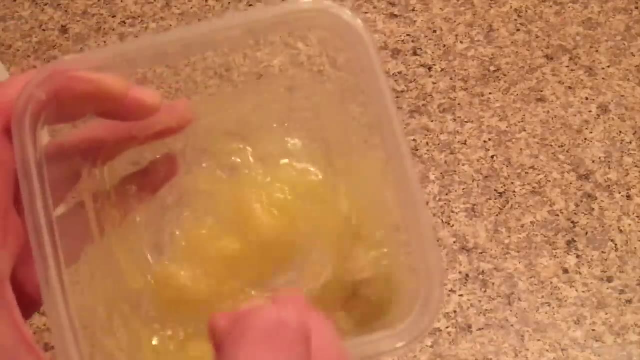 something like that, And it's going to mix it up. It's turning into this like really pretty yellow, which I really do like, And now I'm actually going to put it in the sink and let it sit for about 10 minutes And then I'm going. 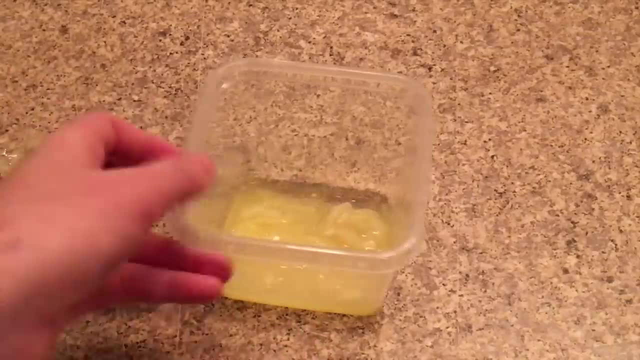 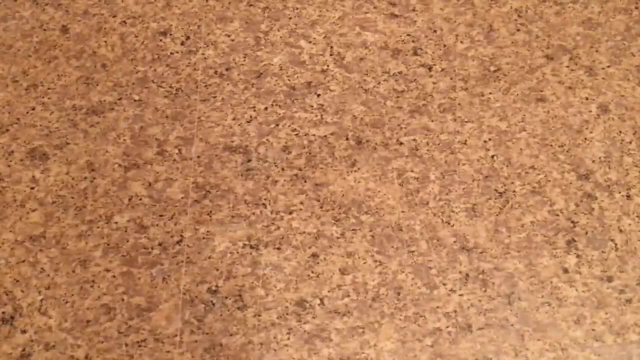 this into the freezer for about an hour, so I'll see you guys in a second. I just noticed there was some pen in me, so I'm gonna wash this off right now. so it's been about an hour and a half and here it is, and it's really bubbly cuz about. 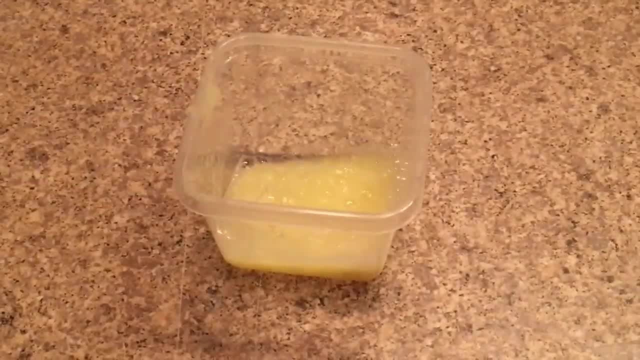 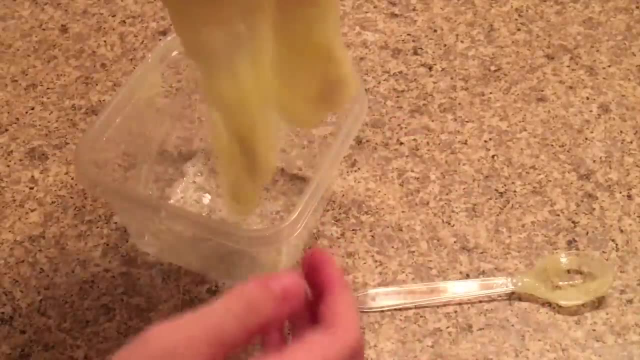 an hour ago. it wasn't really forming really well, so I actually had to mix it a lot, like I mixed it for about 10 minutes and I put it right back in and here it is now and this worked. I am like really shocked right now. this is like so. 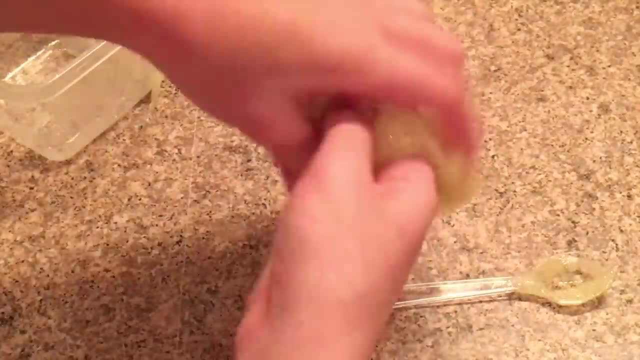 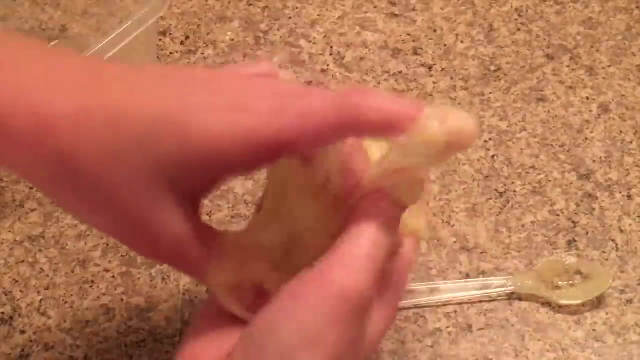 cool. it kind of feels like butter slime, but at the same time it does not. it's like really sickening and it's like it feels really weird, like I don't know how to say how it feels. but like, if you guys want to test this out, I really hope you. 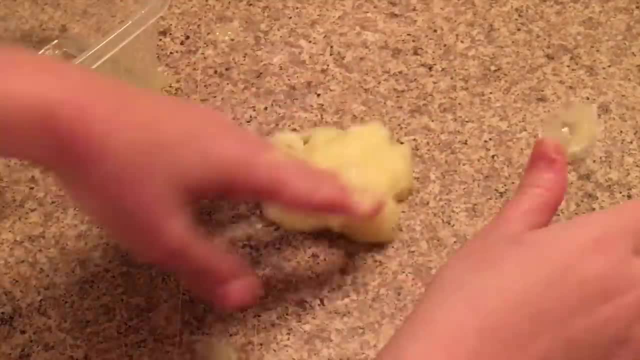 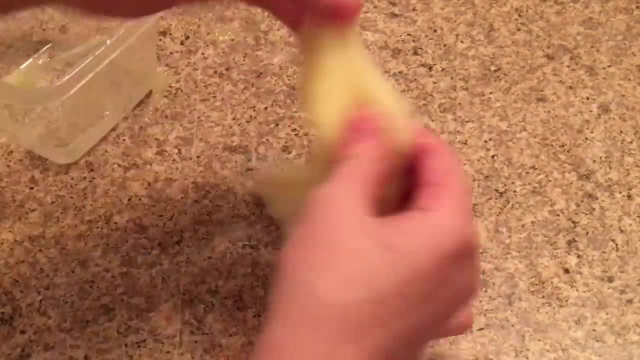 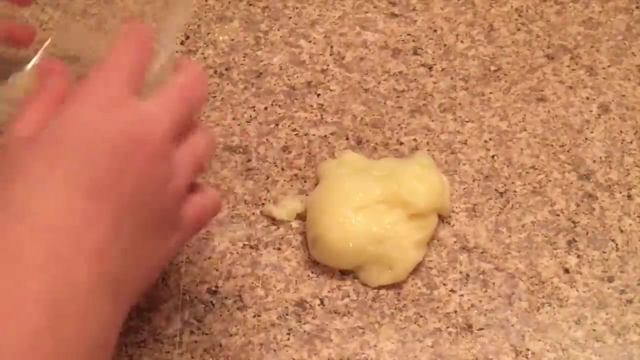 do and like make sure you rip the toilet paper like evenly into like little shreds, and this is just a big win-win. I'm so excited this worked. it has like a weird feeling. so let's move on to the next no glue paper slime recipe I will be showing you guys today. okay, guys, the. 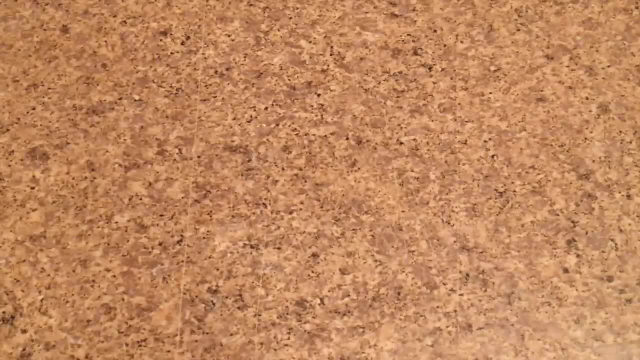 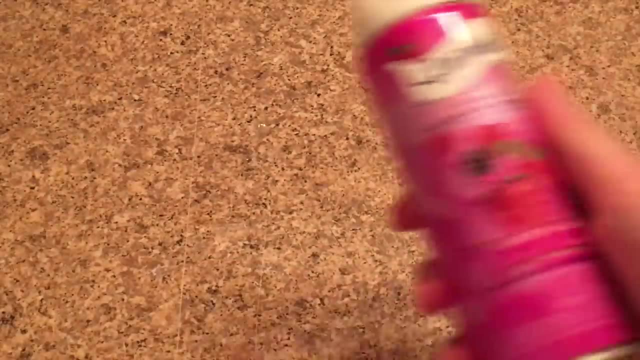 next, no glue paper slime recipe I will be showing you guys today is notebook paper slime. so the ingredients you guys will need to make this slime recipe today is suave kids two-in-one shampoo. you guys will also need some shaving gel or shaving cream. I'm using shaving gel today. 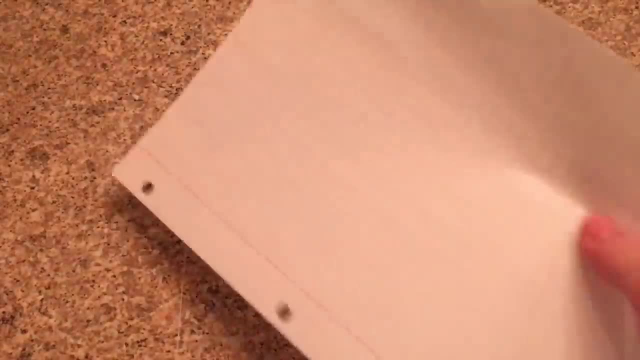 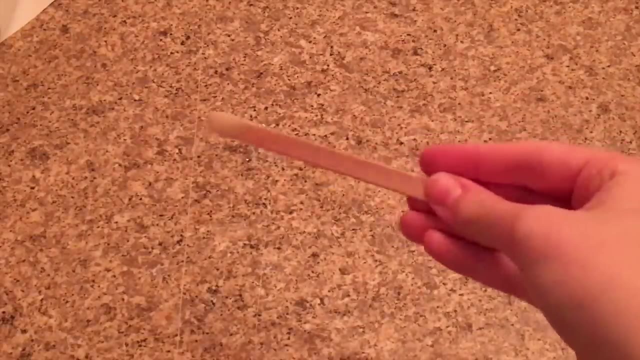 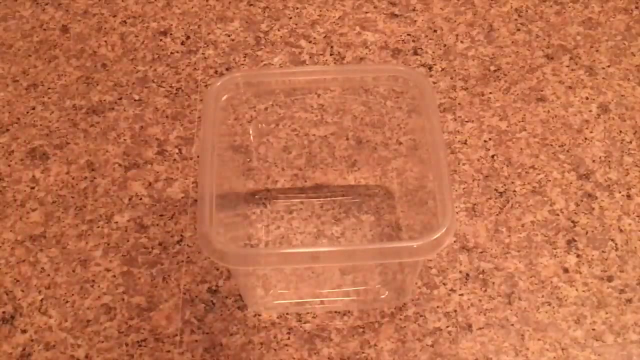 and you guys will need notebook paper and a bowler plate to make your slime in. and, last not least, you guys will need a mixing tool. so first take out your bowl or plate and add in your shaving gel or shaving cream. and here's mine and it: 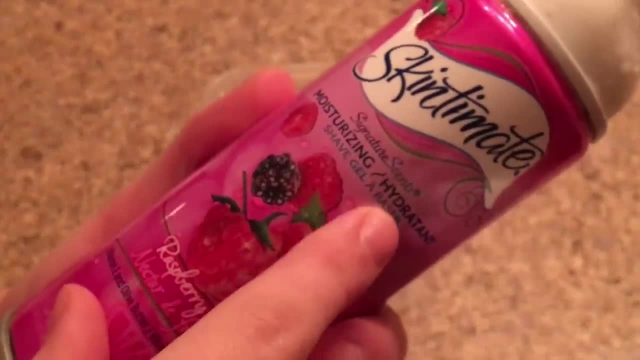 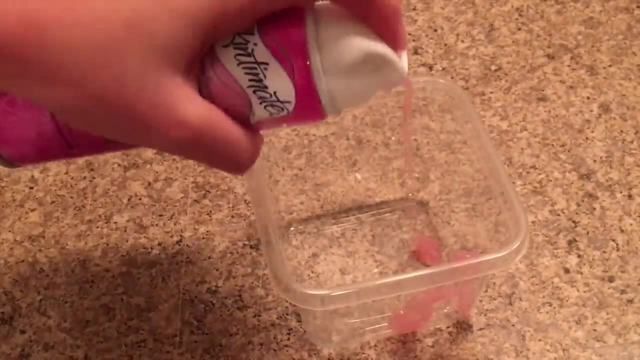 smells like berries. this is the kind I'm using today. it smells so good. I got it like a while ago and it's like good for making fluffy slime and stuff, but now add it into your bowler plate and add as much as you want. I'm actually 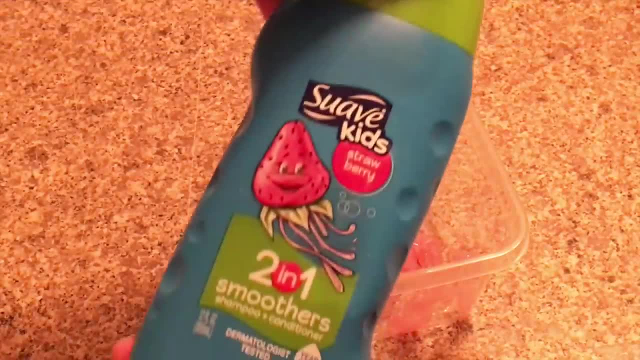 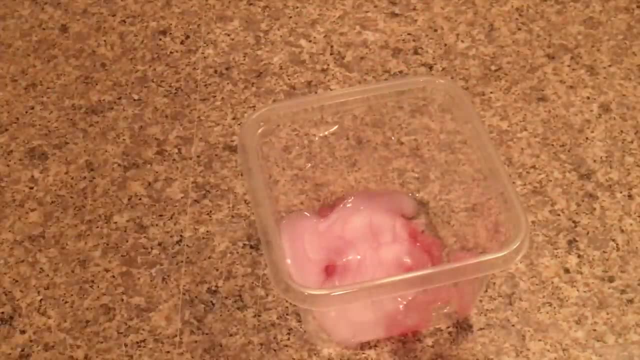 gonna add a lot today so that looks good. and now adding your suave kids two-in-one shampoo. you can also use three-in-one shampoo, like whichever one you want to use, and then give it like a little mix around. it's gonna get like all fluffy. 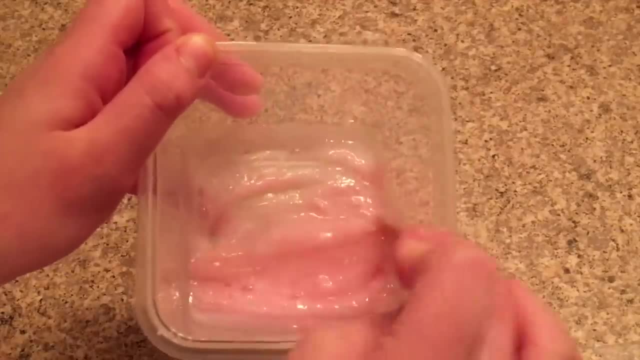 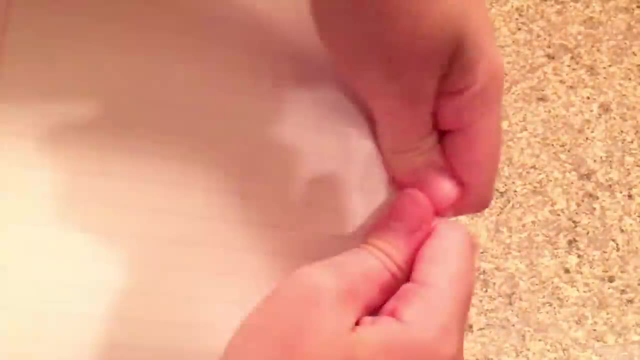 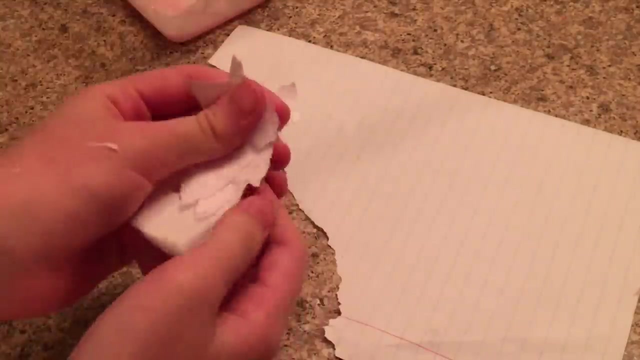 and I'm trying out this recipe for the first time today, same with, like the other ones in this video and like I really hope it works. and now, guys, take out your notebook paper and shred it apart. shred it as much as you did with the toilet paper slime at the beginning of the video. so this is how much I'm. 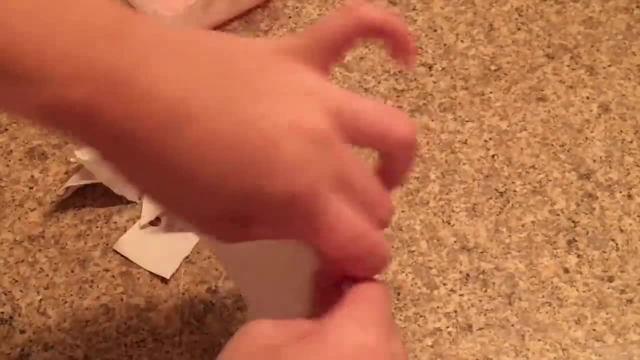 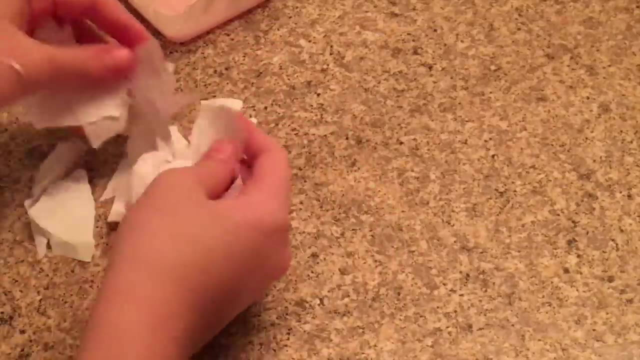 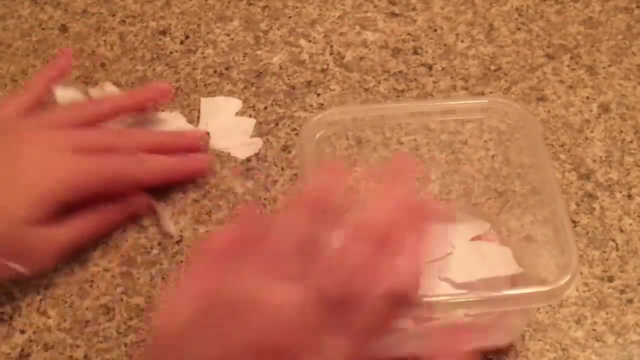 shredding apart and like don't add too much into your like recipe right now, because you don't want it to get like all sickening and it will like go bad and it won't even work. so just go very slowly at adding it. so just gonna add it. 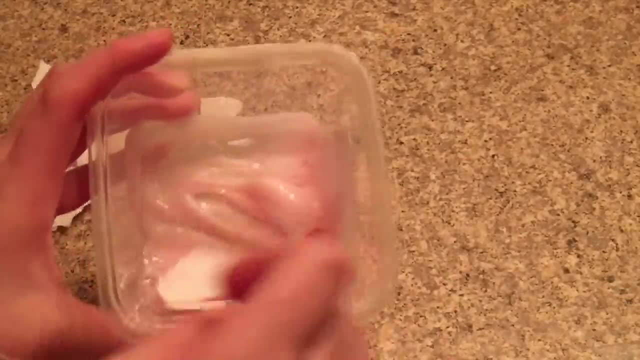 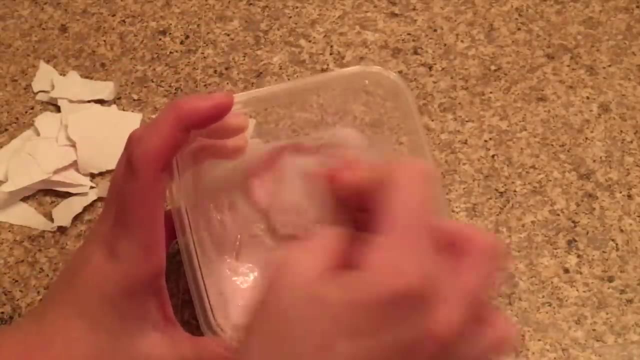 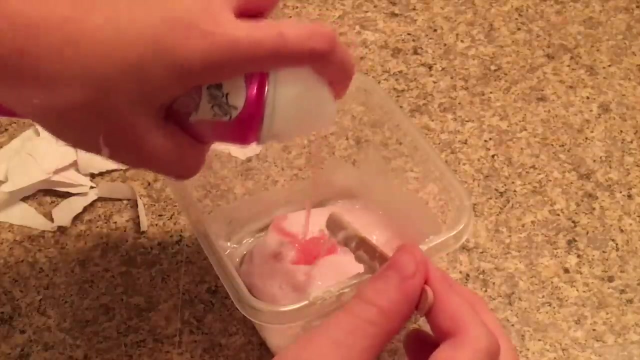 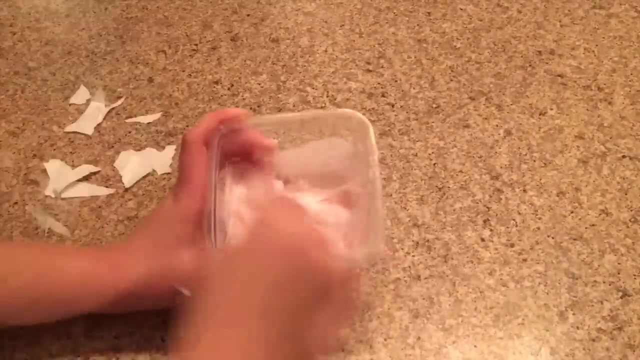 evenly, yeah, and then just get mixing it up and mix like fast, I guess. so like mix really evenly and actually gonna do this as a time-lapse, so I will see you guys in a second. I'm gonna add some shaving gel before I do that. yeah, okay. 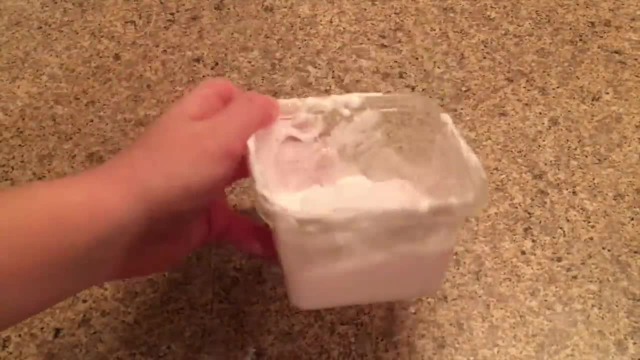 guys. so I've been mixing it for about 10 minutes and here it is okay, guys. so I've been mixing it for about 10 minutes and here it is okay guys. so I've been mixing it for about 10 minutes and here it is, and this is just it being mixed all. 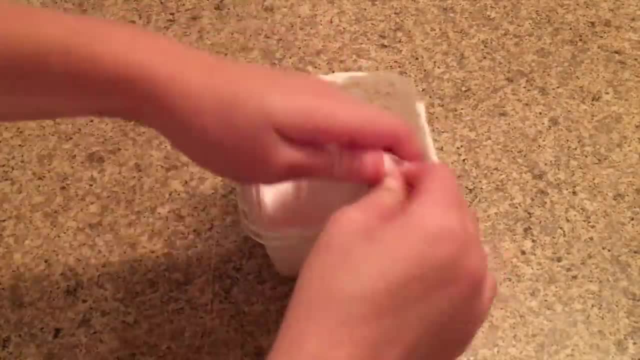 and this is just it being mixed all, and this is just it being mixed all together and it like started forming, but together. and it like started forming, but together, and it like started forming, but like I don't know. it's kind of like I like I don't know, it's kind of like I. 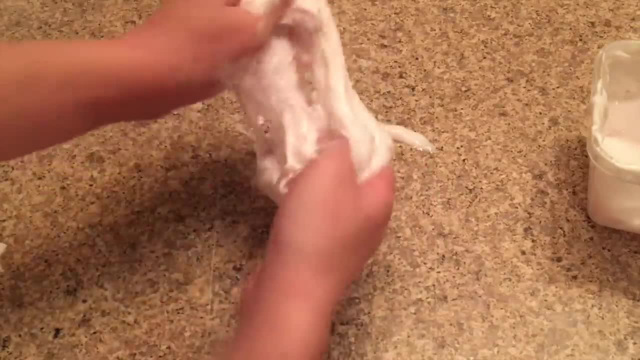 like I don't know. it's kind of like I feel like you should put this in the feel, like you should put this in the feel, like you should put this in the freezer, too, after you're done mixing, but freezer too, after you're done mixing. but 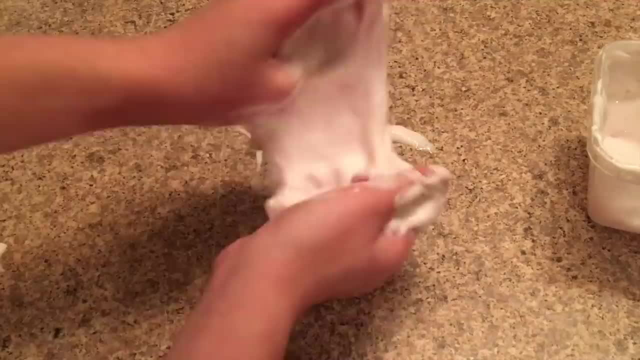 freezer, too, after you're done mixing. but I thought I'd try this without I don't. I thought I'd try this without I don't. I thought I'd try this without I don't know using the freezer or fridge today. know using the freezer or fridge today. 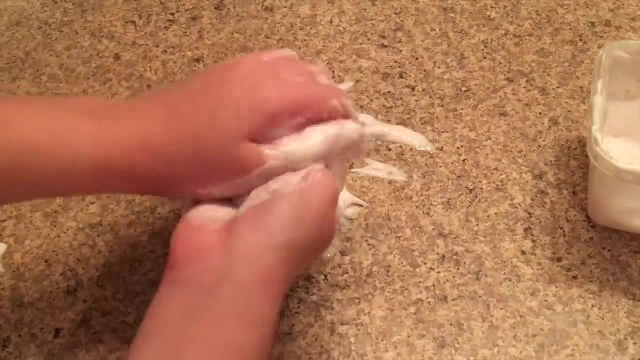 know, using the freezer or fridge today for this recipe, and it's kind of like a for this recipe and it's kind of like a for this recipe and it's kind of like a maybe, maybe cuz I don't know. it's just maybe maybe cuz I don't know, it's just 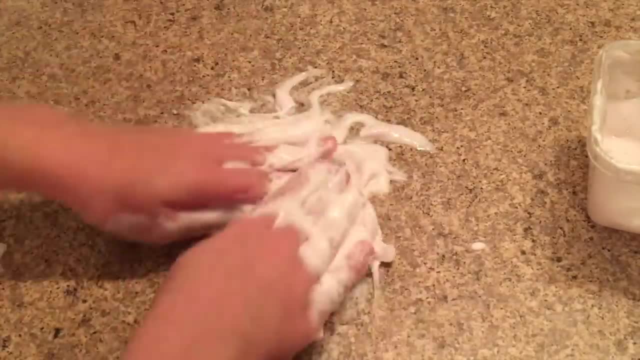 maybe, maybe, cuz I don't know, it's just really sticky and it's not the best. this really sticky and it's not the best. this really sticky and it's not the best. this is really messy too, so try putting it in. is really messy too, so try putting it in. 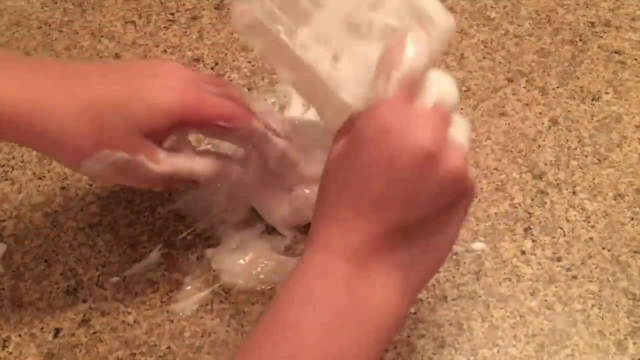 is really messy too, so try putting it in the freezer for like an hour to two, the freezer for like an hour to two, the freezer for like an hour to two hours, but it's actually really clumpy hours. but it's actually really clumpy hours, but it's actually really clumpy, which is odd. it's probably just the. 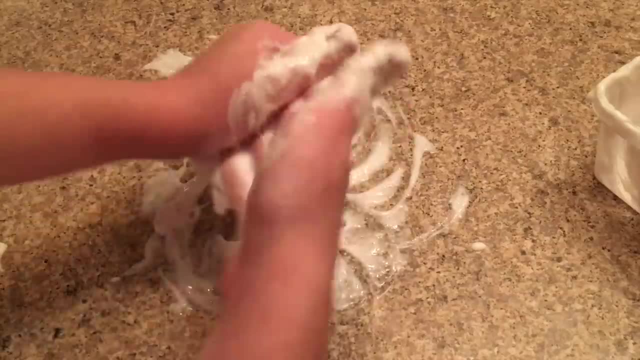 which is odd. it's probably just the which is odd. it's probably just the shaving gel for me come together and it shaving gel for me come together and it shaving gel for me come together and it feels really weird. I don't know, but the feels really weird. I don't know, but the. 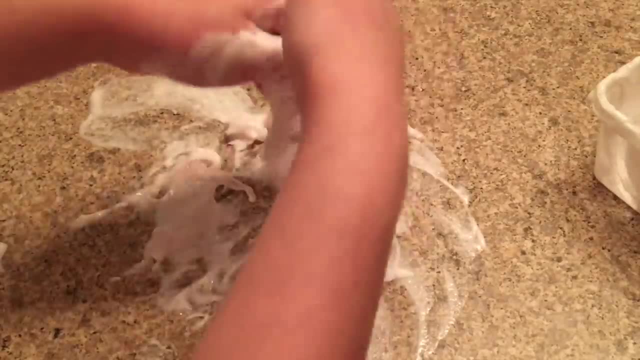 feels really weird. I don't know, but the paper did mix in really well. I'm like paper did mix in really well. I'm like paper did mix in really well. I'm like all the mixing I did like ten minutes, all the mixing, I did like ten minutes. 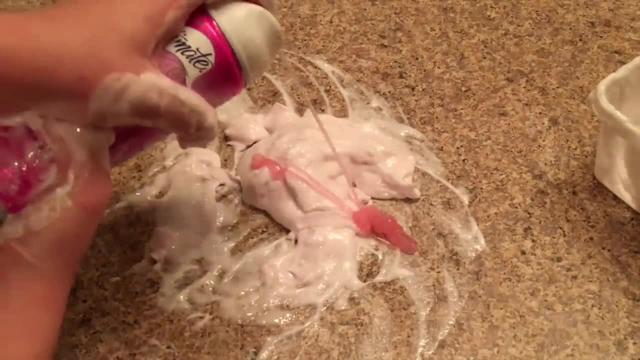 all the mixing I did like ten minutes straight. let's try adding in some more straight. let's try adding in some more straight. let's try adding in some more shaving gel- well, even more messy, but no. shaving gel- well, even more messy, but no. shaving gel. well, even more messy, but no, make sure you clean your mess when you're. 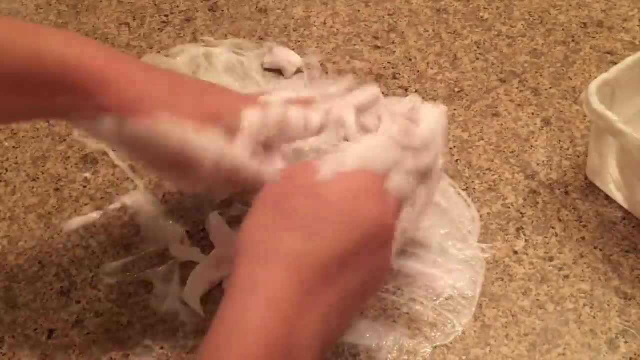 make sure you clean your mess when you're. make sure you clean your mess when you're done. you don't want your parents to get done. you don't want your parents to get done. you don't want your parents to get mad. so this is a maybe, maybe. so let's. 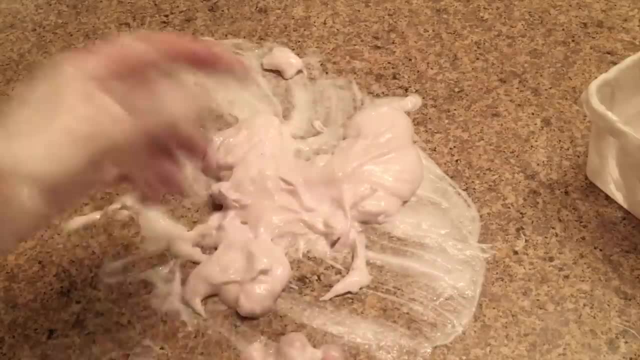 mad. so this is a maybe, maybe. so let's mad. so this is a maybe, maybe. so let's move on to the next. no glue paper slime. move on to the next. no glue paper slime. move on to the next. no glue paper slime recipe. I'll be shooting guys today, okay. 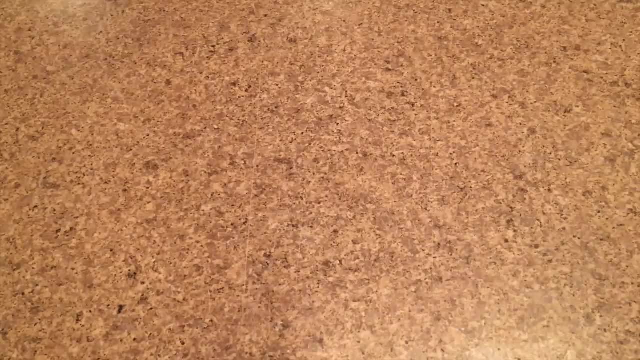 recipe: I'll be shooting guys today. okay recipe, I'll be shooting guys today. okay guys. so the last and final. no glue guys. so the last and final. no glue guys. so the last and final. no glue paper. sign my speed, I will be testing paper. sign my speed, I will be testing. 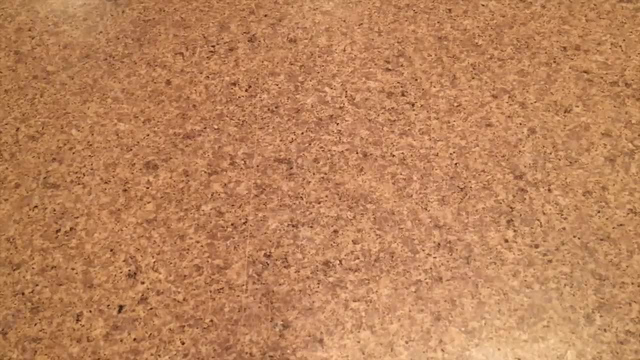 paper sign my speed I will be testing. today is wrapping paper slime, so the today is wrapping paper slime, so the today is wrapping paper slime. so the ingredients you guys will need to make ingredients you guys will need to make ingredients you guys will need to make this slime recipe is dish soap I'm using 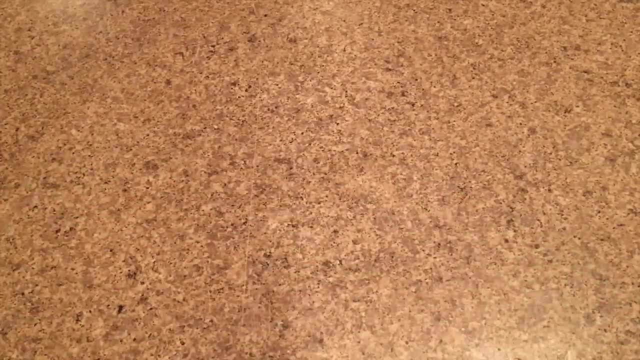 this slime recipe is dish soap. I'm using this slime recipe is dish soap. I'm using Ajax fish soap. the next thing you guys Ajax fish soap, the next thing you guys Ajax fish soap- the next thing you guys will need is wrapping paper, and this will need is wrapping paper and this. 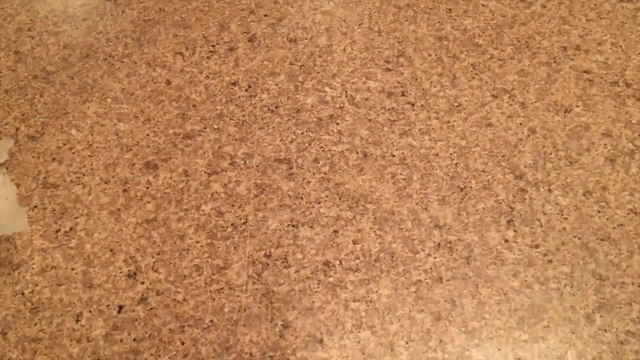 will need is wrapping paper, and this one's really glittery, really pretty you one's really glittery, really pretty you one's really glittery, really pretty. you guys will also need a bowler plate. to guys will also need a bowler plate. to guys will also need a bowler plate to make your slime in. and last but not, 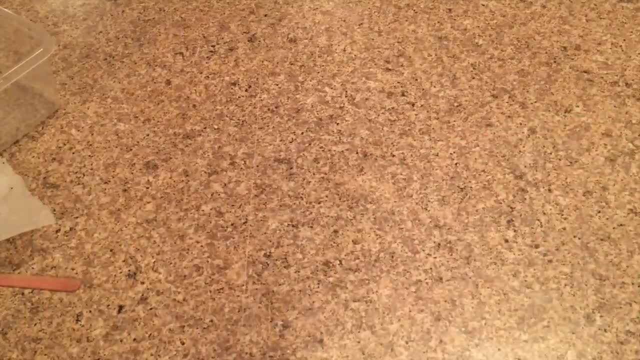 make your slime in. and last but not, make your slime in. and last but not least, you guys will need a mixing tool. so first take out your bowl or plate. so first take out your bowl or plate. so first take out your bowl or plate and you guys will have to add in your 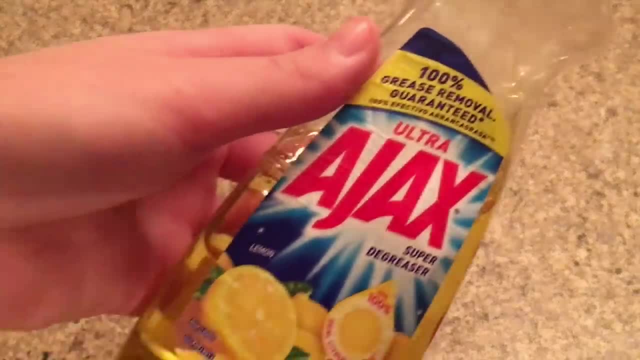 and you guys will have to add in your and you guys will have to add in your dish soap. you guys can use like any kind dish soap. you guys can use like any kind dish soap. you guys can use like any kind of using this one today and add as much. 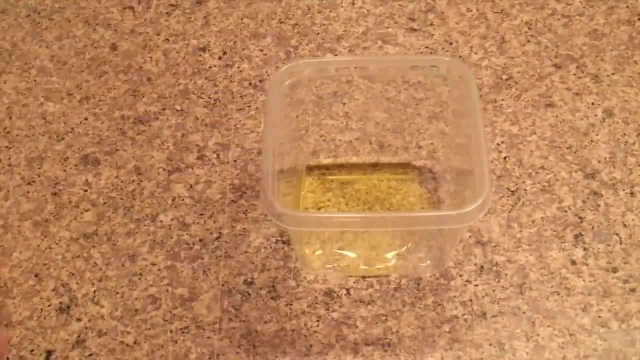 of using this one today and add as much of using this one today and add as much as you want in there. so I'm gonna add as you want in there. so I'm gonna add as you want in there. so I'm gonna add about this much, not too much, I don't. 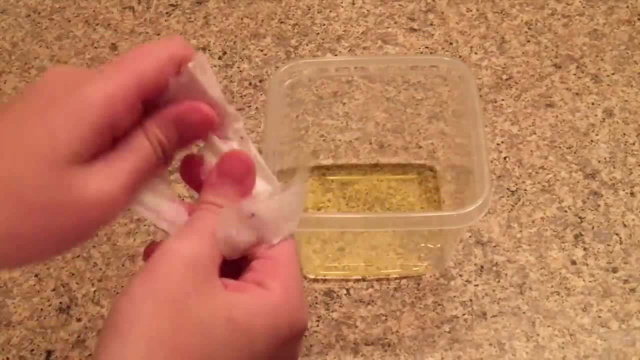 about this much, not too much. I don't about this much, not too much. I don't want to waste it all. and then you guys want to waste it all, and then you guys want to waste it all, and then you guys will add in your wrapping paper: and I'm 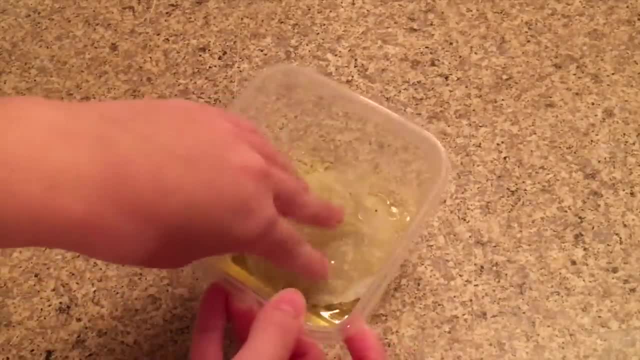 will add in your wrapping paper and I'm will add in your wrapping paper and I'm actually gonna add it into like big, actually gonna add it into like big, actually gonna add it into like big pieces, because I want to see what pieces, because I want to see what. 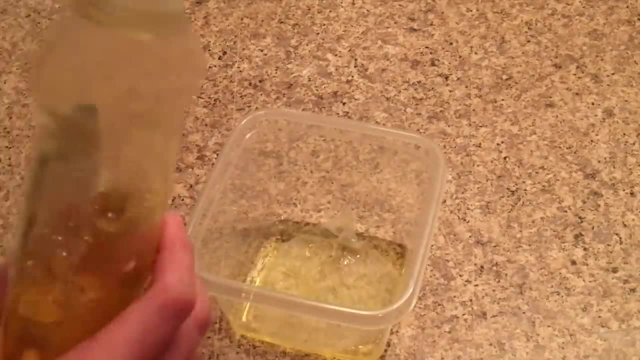 pieces because I want to see what happens to it. I'm gonna do it like that happens to it. I'm gonna do it like that happens to it. I'm gonna do it like that. I'm just gonna add some more dish soap. I'm just gonna add some more dish soap. 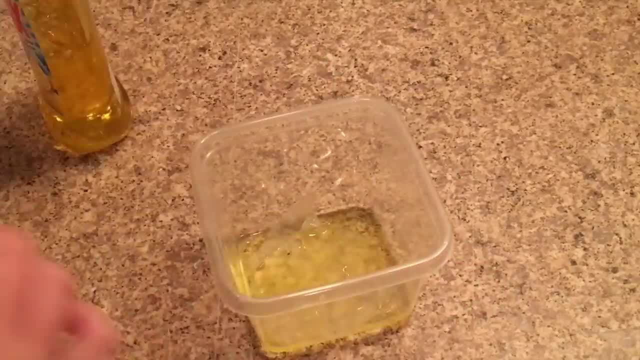 I'm just gonna add some more dish soap on top, kind of like layering it. I guess on top, kind of like layering it. I guess on top, kind of like layering it. I guess you can say I'm just gonna pat it down. you can say I'm just gonna pat it down. 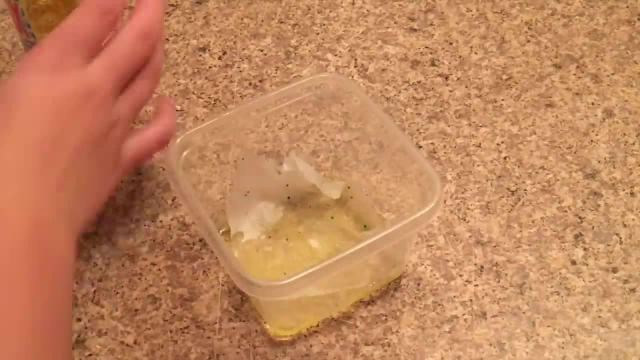 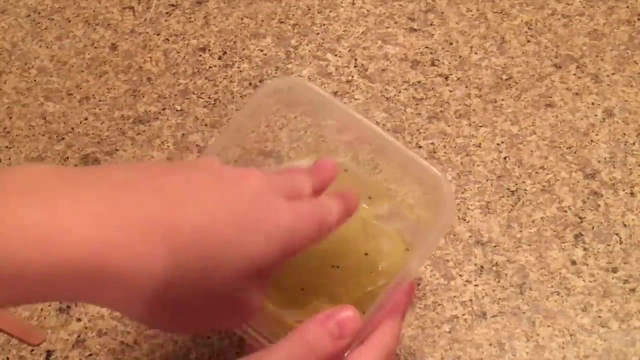 and add another piece, add more notice, and add more notice and add more notice. same process over and over again, and same process over and over again, and same process over and over again. and then I'm gonna like mix it up with my, then I'm gonna like mix it up with my. 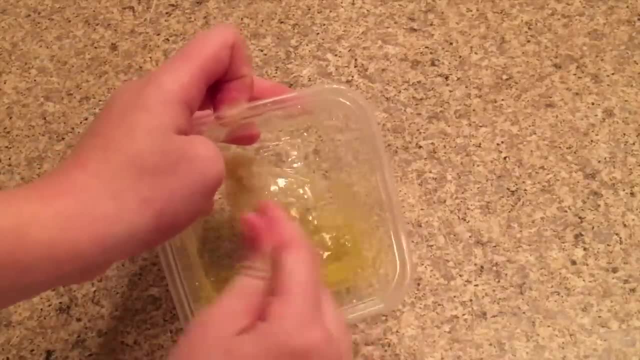 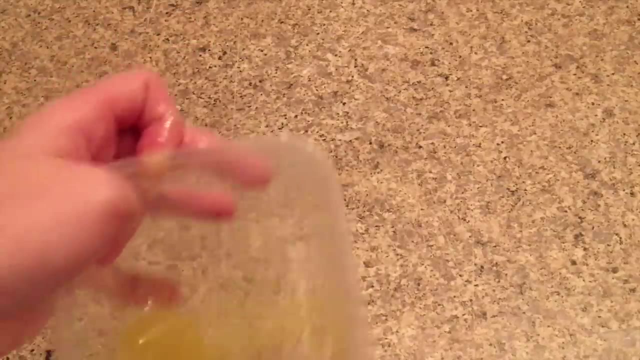 then I'm gonna like mix it up with my mixing tool and this is really weird. but mixing tool and this is really weird. but mixing tool and this is really weird. but like all the soap dissolved into like like all the soap dissolved into like like all the soap dissolved into like the wrapping paper, and I got all stuck. 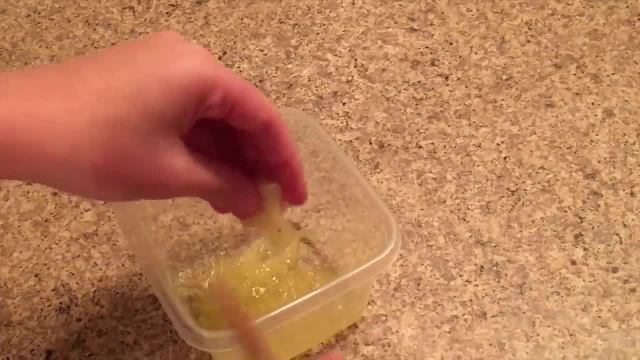 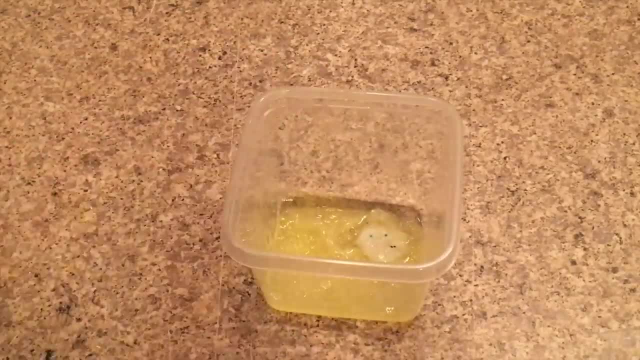 it's turning into a weird color and stuff. it's turning into a weird color and stuff. I don't know. this one's just really. I don't know. this one's just really I don't know. this one's just really cool. and now you guys gonna put this. 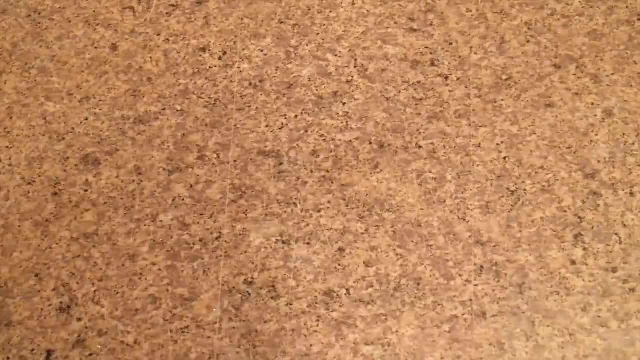 cool. and now you guys gonna put this cool, and now you guys gonna put this into the freezer for about an hour. so I into the freezer for about an hour, so I into the freezer for about an hour. so I will see you guys in a second. so it's. 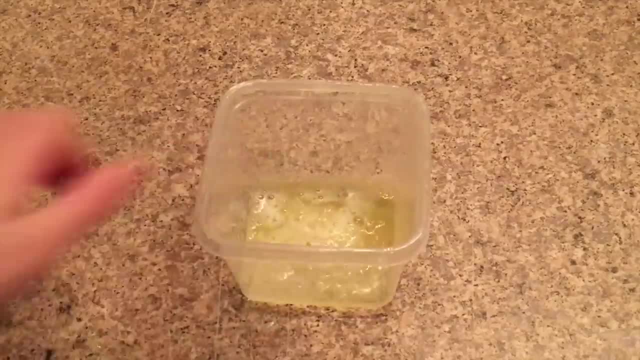 will see you guys in a second. so it's will see you guys in a second. so it's been about an hour and here it is. it's been about an hour and here it is. it's been about an hour and here it is. it's really soapy because when I took it out, 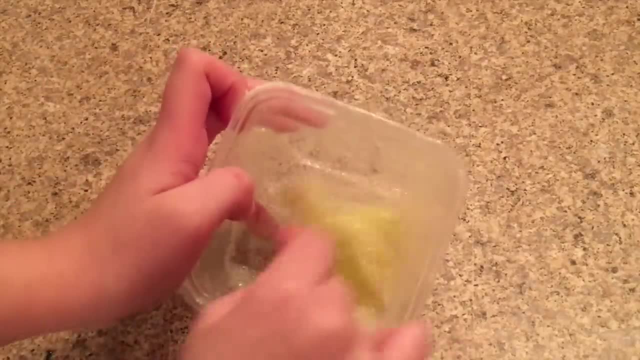 really soapy because when I took it out- really soapy because when I took it out and mixed a little bit to see what and mixed a little bit to see what and mixed a little bit to see what, happened what- this is really cool guys. happened what? this is really cool guys. 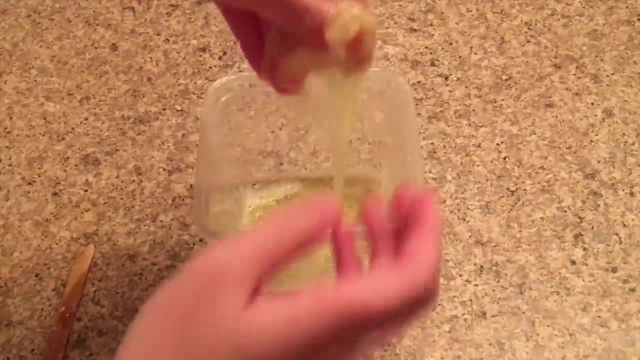 happened what? this is really cool guys. this is like water slime, I don't know. this is like water slime, I don't know. this is like water slime, I don't know, but the paper is like kind of making it. but the paper is like kind of making it. 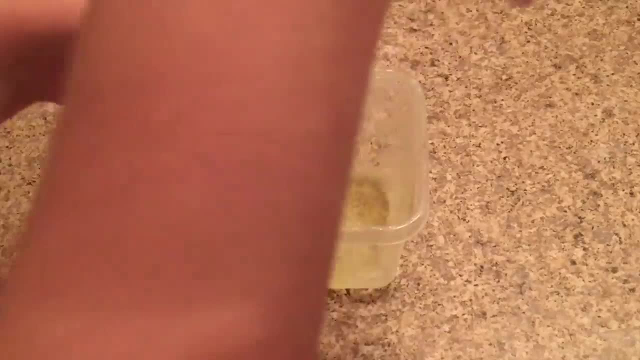 but the paper is like kind of making it kind of like a butter slime, but at the kind of like a butter slime, but at the kind of like a butter slime, but at the same time like look at this, sorry, my same time like look at this, sorry, my. 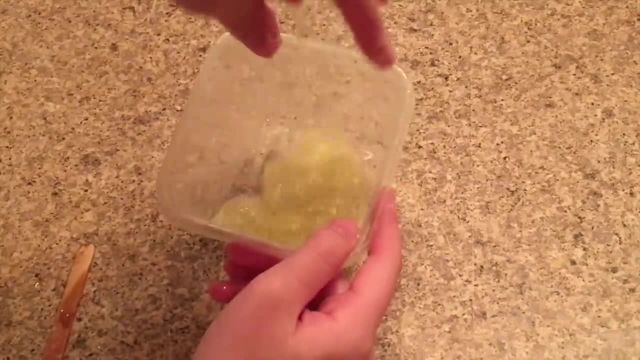 same time like look at this, sorry, my hands like in the way, but it's it's kind hands like in the way, but it's it's kind hands like in the way, but it's it's kind of like I don't know what to call it. 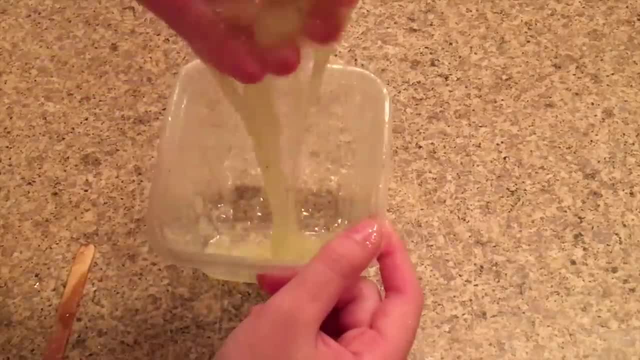 of like I don't know what to call it. of like I don't know what to call it. maybe jelly slime, like the it's kind of. maybe jelly slime like the it's kind of. maybe jelly slime like the it's kind of doesn't feel watery. some you get it at. 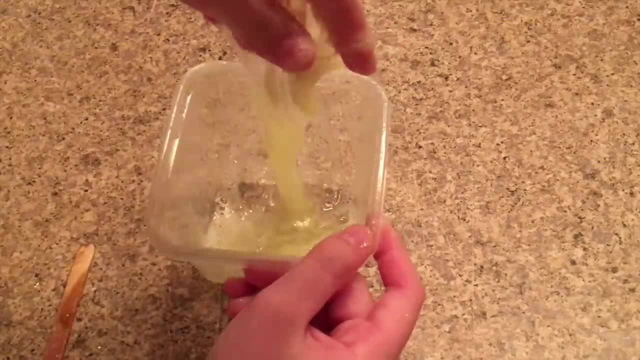 doesn't feel watery. some you get it at doesn't feel watery. some you get it at like the Dollar Tree and like the toy, like the Dollar Tree and like the toy, like the Dollar Tree and like the toy section. it's really watery and like. 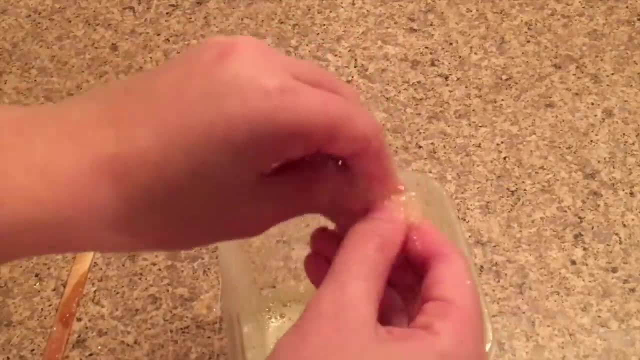 section it's really watery and like section it's really watery and like water-based. I guess you can say and like water-based. I guess you can say and like water-based. I guess you can say and like: the wrapping paper is making it like. the wrapping paper is making it like. 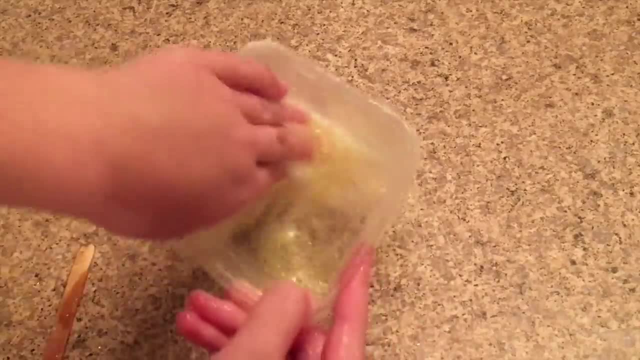 the wrapping paper is making it like more thick, which is really cool. this more thick, which is really cool. this more thick, which is really cool. this one's like a maybe, maybe. I guess you one's like a maybe, maybe. I guess you one's like a maybe, maybe. I guess you guys might like this. maybe not, but you. 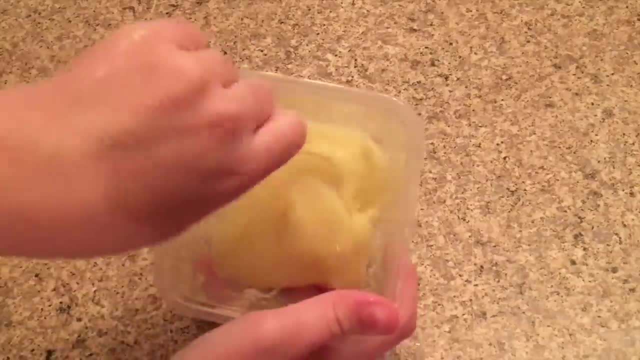 guys might like this, maybe not, but you guys might like this, maybe not. but you know what I like this one, so thank you. know what I like this one, so thank you. know what I like this one, so thank you, guys, so much for watching this video. guys, so much for watching this video. 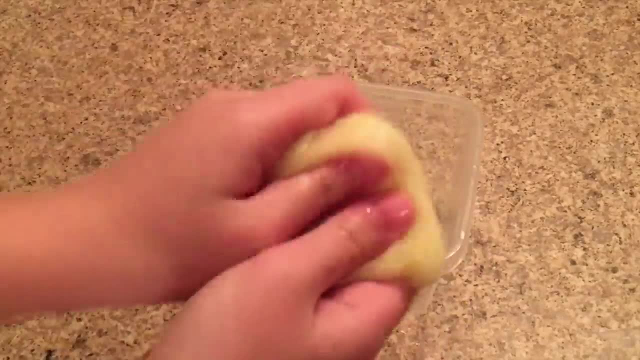 guys, so much for watching this video today. this is my first one. this is the today. this is my first one. this is the today. this is my first one. this is the toilet paper sign. this one was a big toilet paper sign. this one was a big toilet paper sign. this one was a big win-win. I really want you guys to try it.